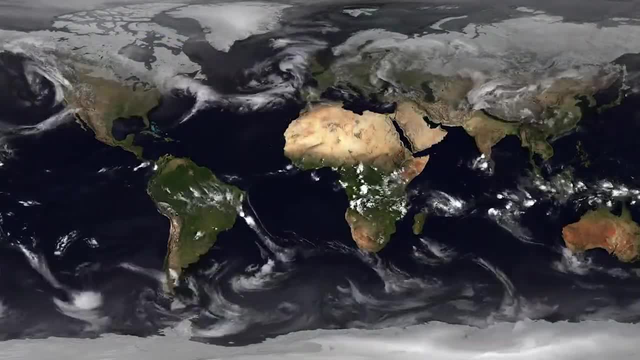 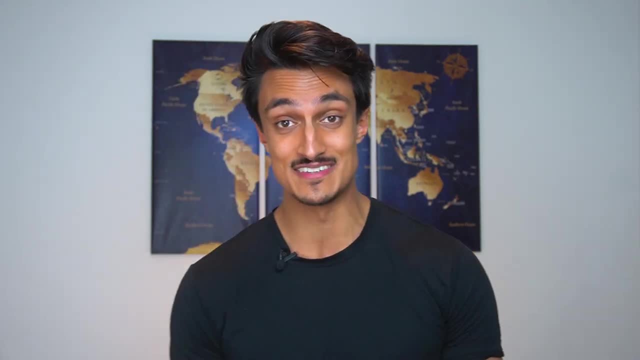 climate are expressions of the movement of energy through the atmosphere and ultimately, all that energy comes from the sun. If you live in the UK, most of the time it's hard to tell if the sun's even there, and I promise you it's working away in the background providing the heat which evaporates. 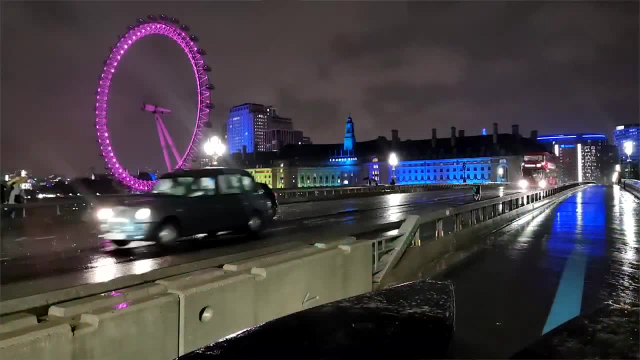 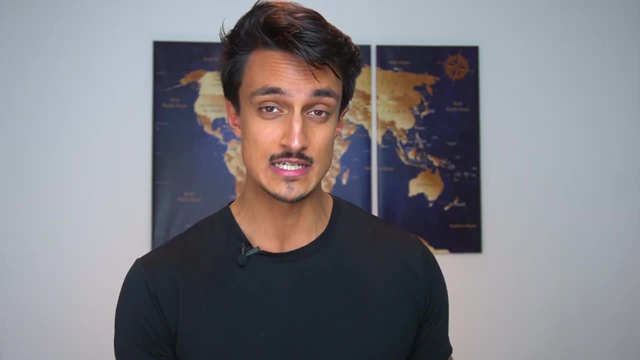 the water which forms the clouds and rain which perpetually cover the British skies. But while both weather and climate are confined to the atmosphere, the energy which drives them is not. In addition to the atmosphere, there are four other parts of our Earth through. 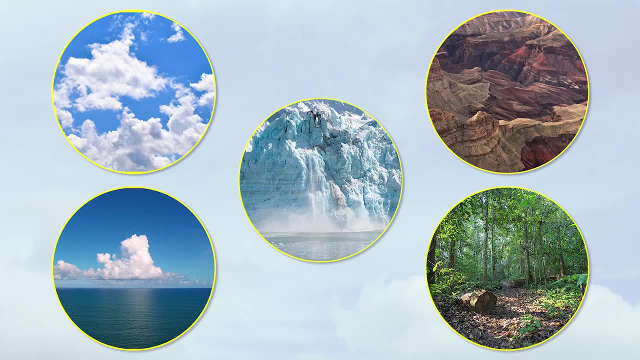 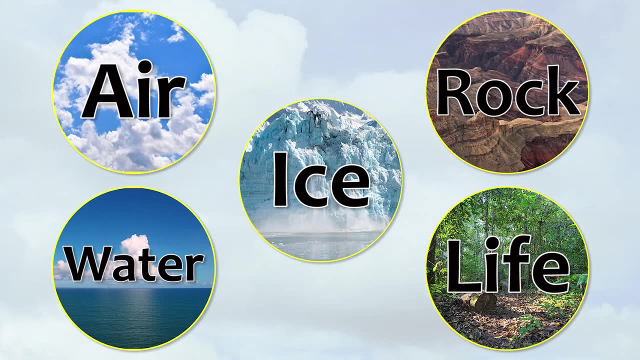 which this energy moves, and together they create our climate. Air, water, ice, rock and life. These five parts of our planet make up the atmosphere, And the atmosphere is the most important part of the atmosphere because it's where we make up the climate system. 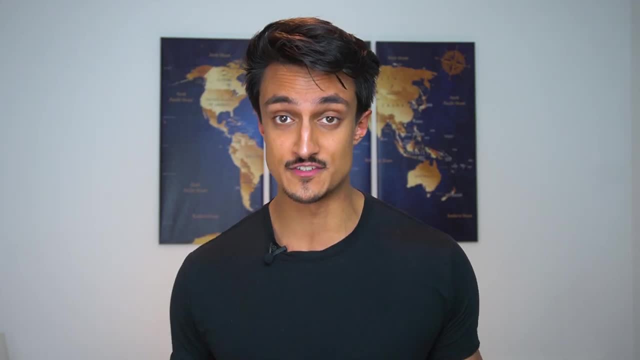 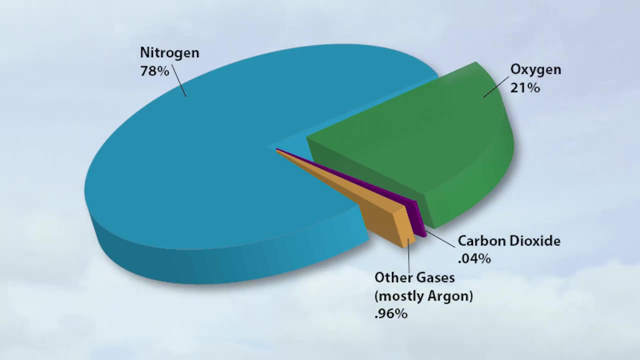 So let's start with air, the atmosphere. As we've just seen, this is where both weather and climate occurs, and it's nearly entirely composed of gases, the most important of which, at least as far as the climate is concerned, are the greenhouse gases, which control the amount of energy. 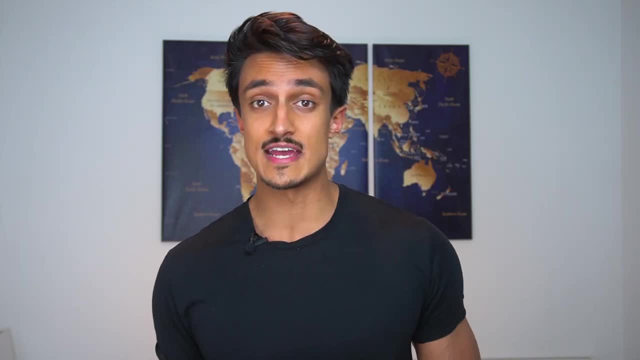 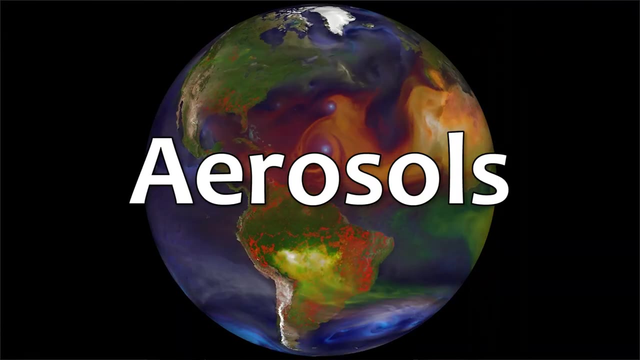 retained by the atmosphere, But the atmosphere also contains ice crystals and water droplets, which make up clouds, as well as tiny dust-like particles called aerosols. These are also important for the climate, since both clouds and aerosoles can reflect sunlight into space. 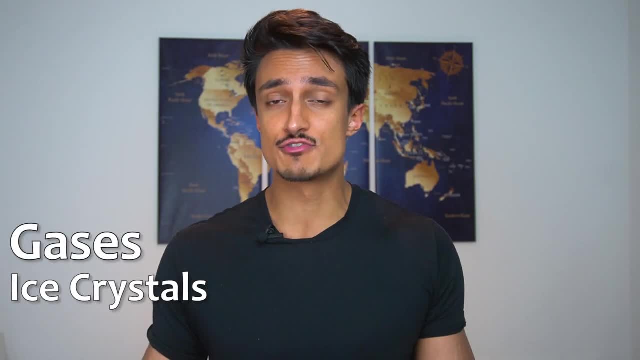 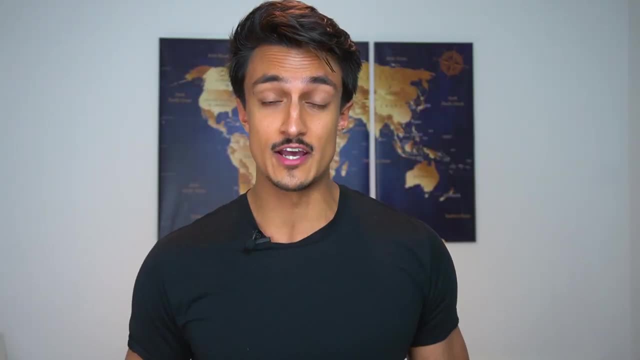 and the former can trap heat. These gases – ice crystals and water droplets – are constantly in motion as vast amounts of energy is transferred above us. Normally, the only time we're aware of this movement is when the wind blows, but if you've ever seen a 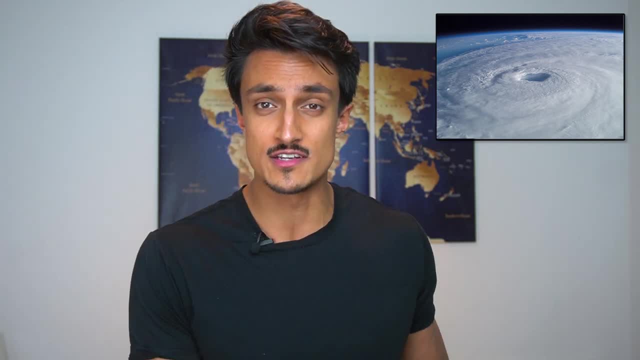 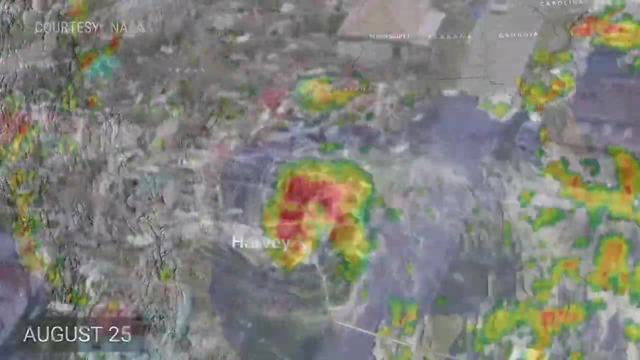 tropical storm on the news or first-hand, you'll have witnessed the massive amount of energy that the atmosphere can carry. Indeed, like each other, tropical storms can release the equivalent of thousands of atomic bombs of energy over their lifetimes, levelling cities and dropping huge quantities of water. 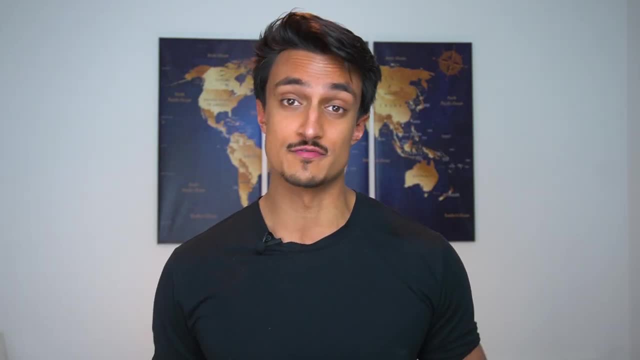 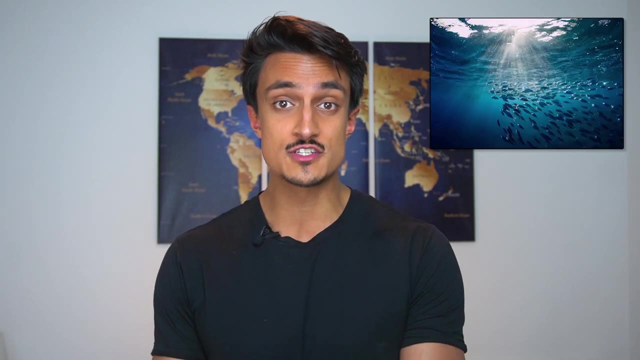 from the sky. And that brings us on to the second component of the climate system: water, or, to use its scientific term, the hydrosphere. This includes all the world's oceans, lakes, rivers, swimming pools and bath water. Now, obviously, the oceans make up the main component here, accounting. 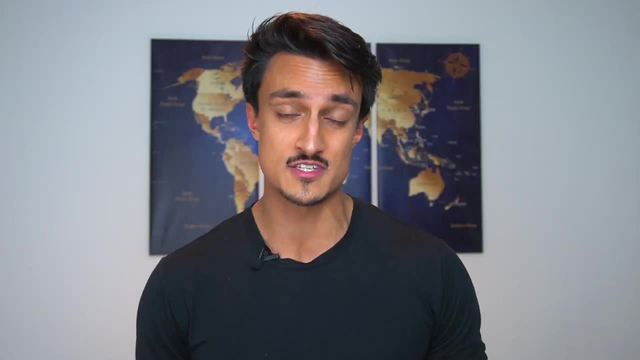 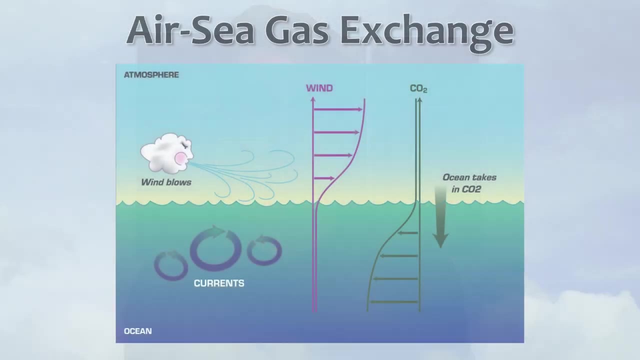 as they do for 70% of the Earth's surface and 97% of the world's water, though, judging by my water bills, my house comes a close second. The oceans can exchange gases with the atmosphere and store a huge amount of energy. Just think. 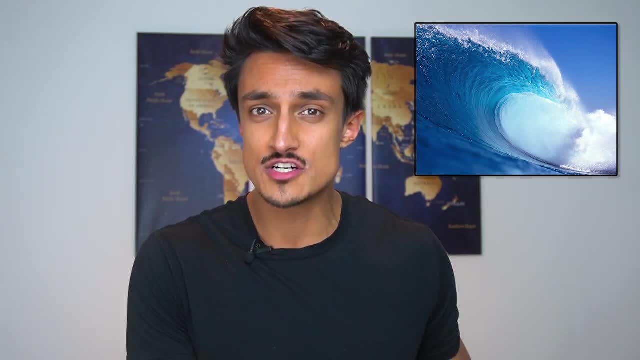 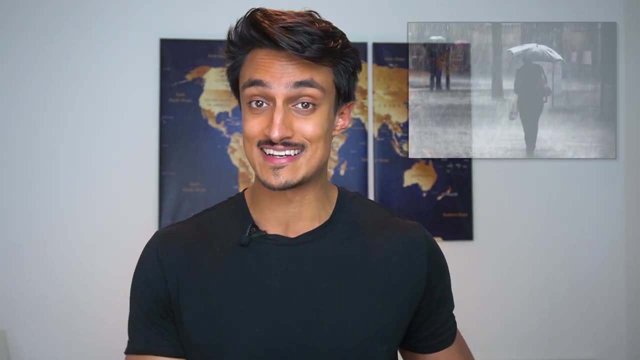 how even a small wave can knock you off your feet, and then imagine how much more energy is stored in all that water moving around our planet. Oceans are also the primary source for most of the rain. that keeps those of us here in the UK in a perpetual state of sarcasm and self-loathing. 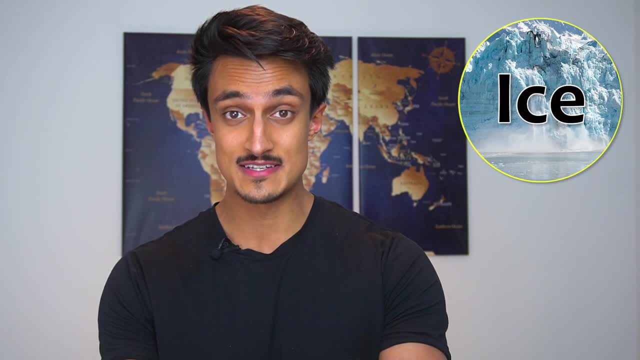 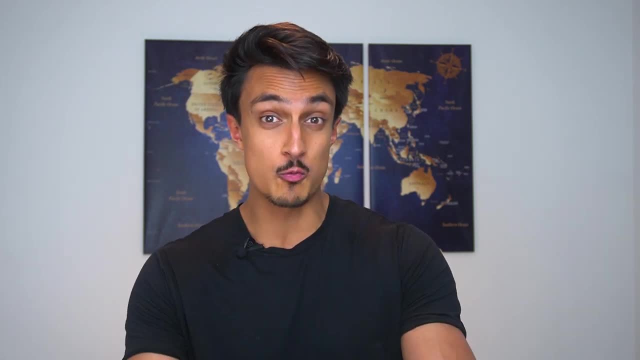 The next component is closely related to the last ice. This part of the climate system is called the cryosphere and it's comprised of 33 million cubic kilometres of ice, which would make one heck of an ice cube or a really big mojito. The energy involved in the melting and freezing of ice and the 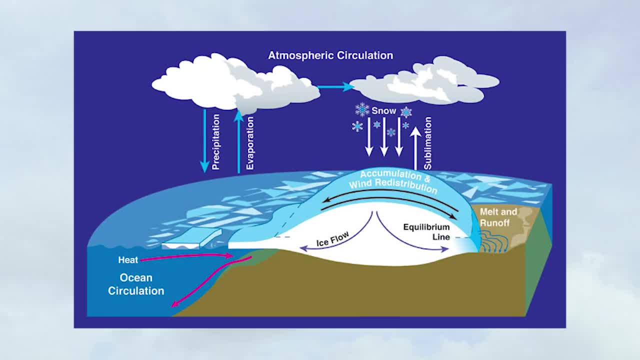 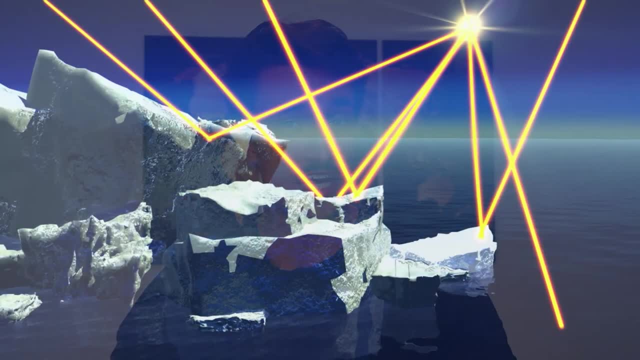 exchange of water with both the hydrosphere and the atmosphere are important functions of the climate system, and the bright surface of both ice and snow plays an important role in reflecting solar energy into space, second only to the blinding surface of Jeff Bezos'. 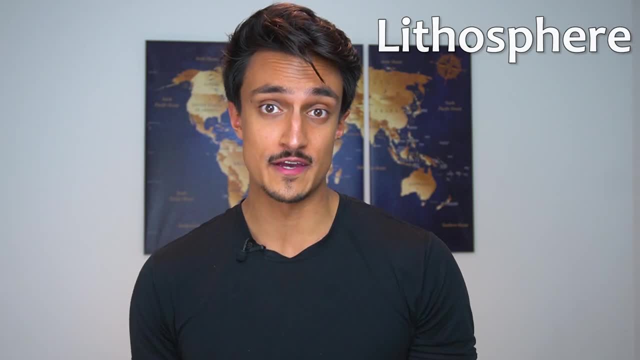 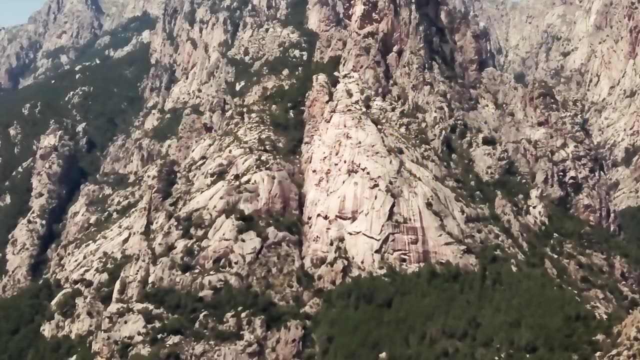 massive head. Next up we have rock: the lithosphere. Surprisingly, the most important part of the lithosphere to the climate system is the land surface. The type of rock that the surface is made of determines how well it will absorb and transfer heat to the rest of the climate system. The shape of the land – the hills, valleys and mountains – also plays an important role through its ability to change how the atmosphere circulates. For example, the Himalayas create the movement of air, responsible for the Asian monsoon. The lithosphere can also affect the composition of the atmosphere by spewing gases out of 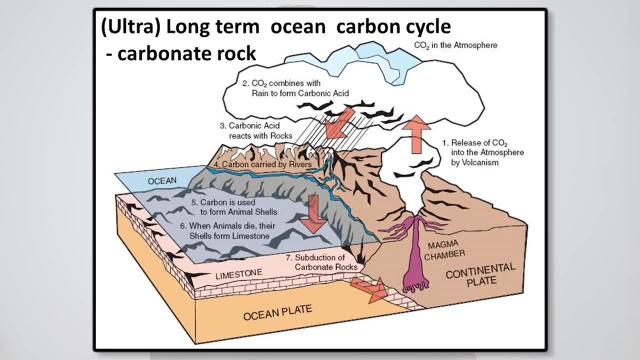 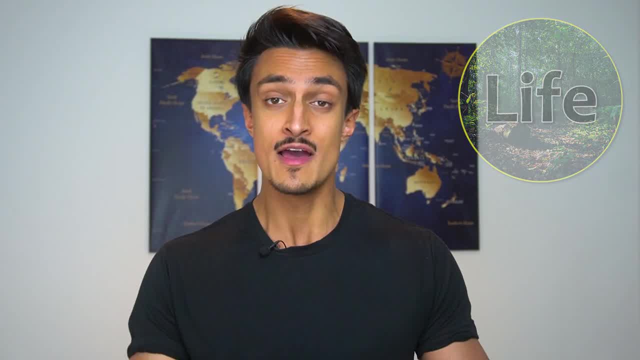 volcanoes and by chemically reacting with rainwater to suck carbon dioxide out of the atmosphere. And that brings us to the final component: life, or, to use its scientific name, the biosphere. This part of the climate system incorporates all living things, from an ant to a blue whale. 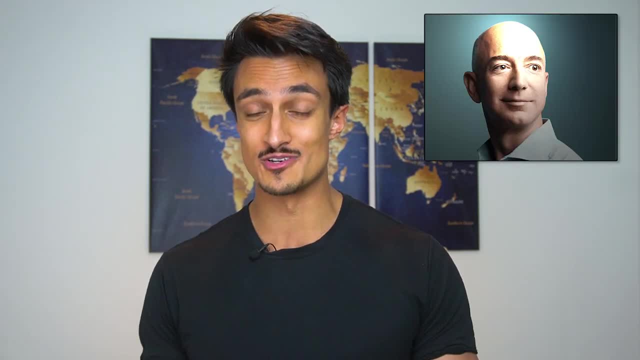 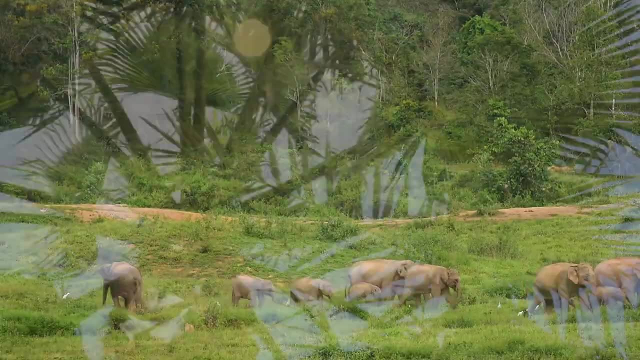 from a salad leaf to a palm tree and from a bacterium to Jeff Bezos and his massive shiny head. Compared to the oceans and atmosphere, the energy contained and transported within the biosphere is tiny, And yet we are all apart. 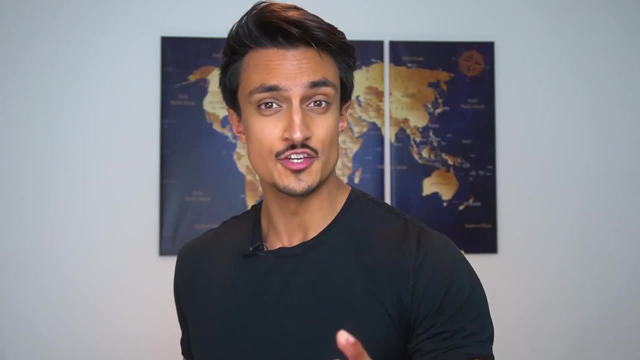 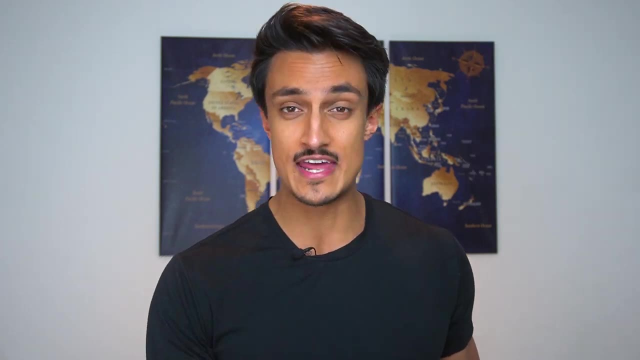 Let's start this energy transfer. Every second that you are alive, you use energy that you got from your food, And unless your food came from another galaxy, your lunch originally got that energy from the sun, either via photosynthesis, if it was a plant, or by eating a plant itself.